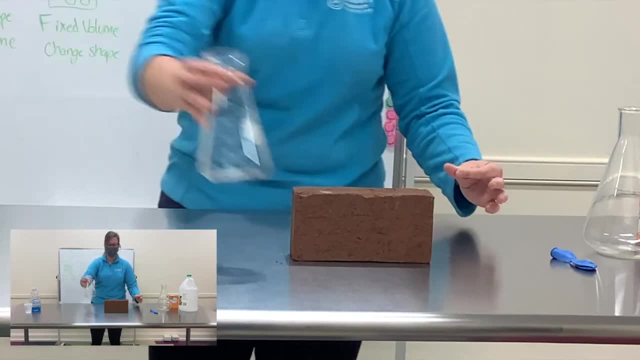 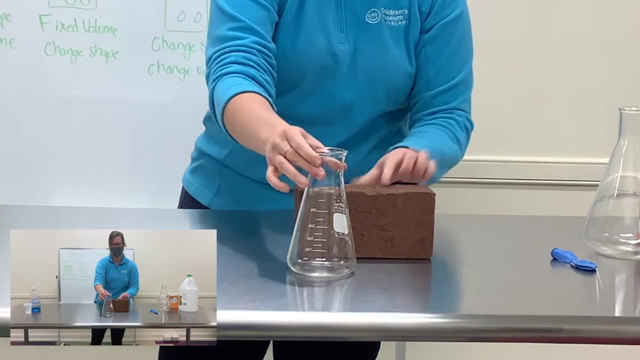 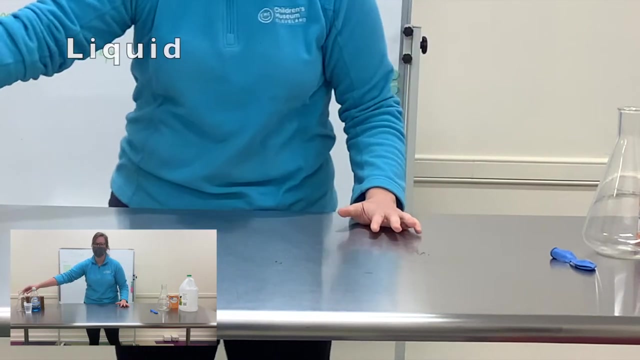 is not going to matter. It's not going to change And its shape is also not going to change. If I try to put my brick into this container, it is not changing to fit inside And that makes it a solid. Our next state of matter is liquids, So I'm going to give it my container again. 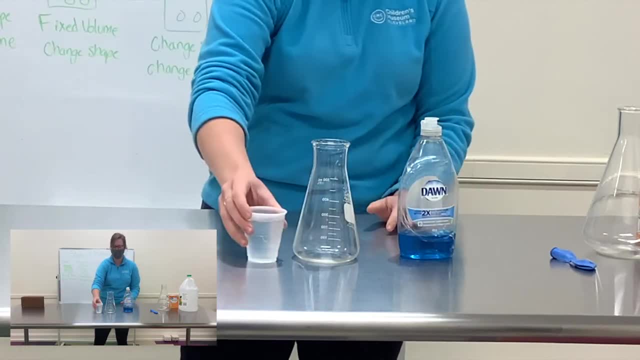 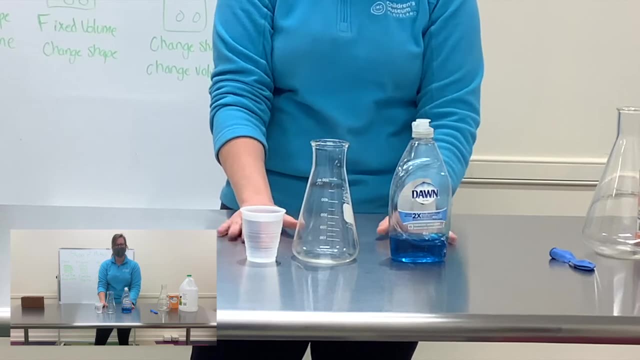 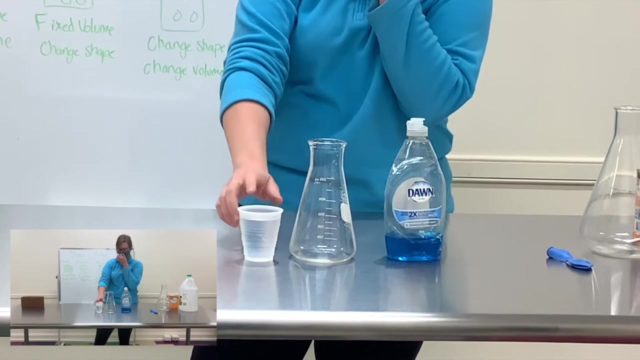 And here I have two types of liquid. I have water and I have soap. Both are liquids you might be familiar with. A liquid has the same volume, So I'll always have this amount of soap, even if I pour it in here, And I'll always have this amount of water, even if I pour it in here. 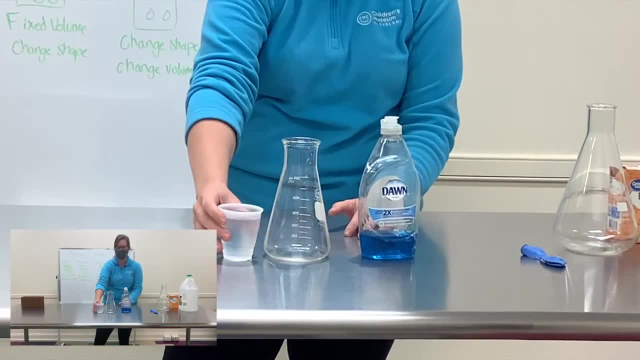 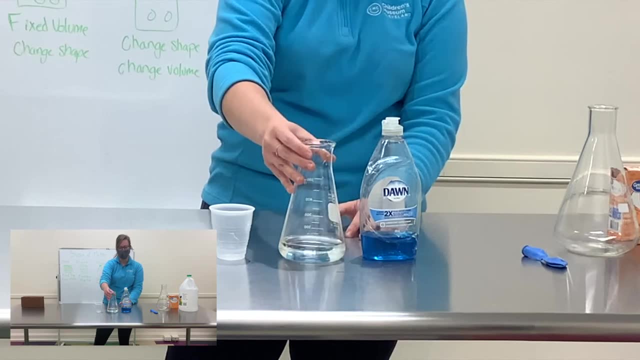 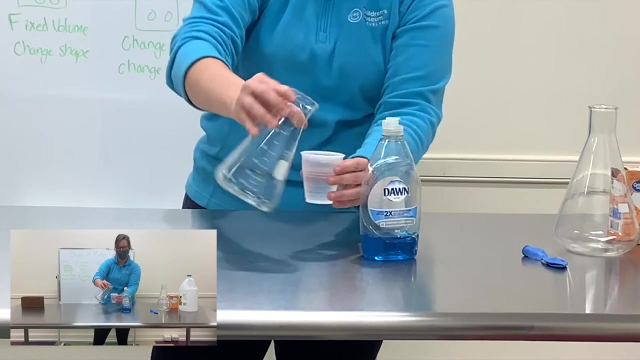 But different than the brick, they will change their shape. So if I pour my water in here, it has now spread out and taken the shape of my container. Now my water pours pretty quickly. It pours very fast. That means it is not very viscous, which is almost like a fancy science term for thick. 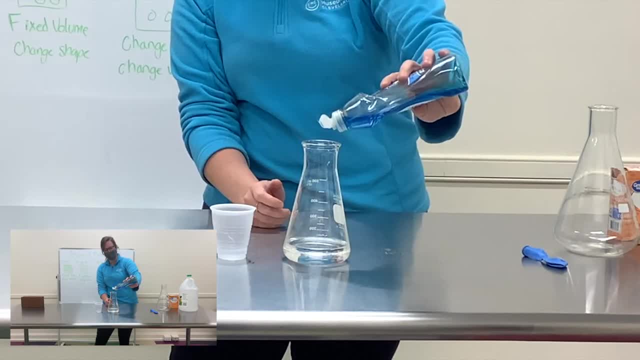 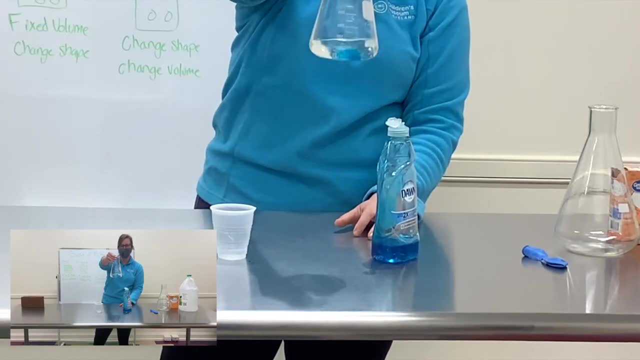 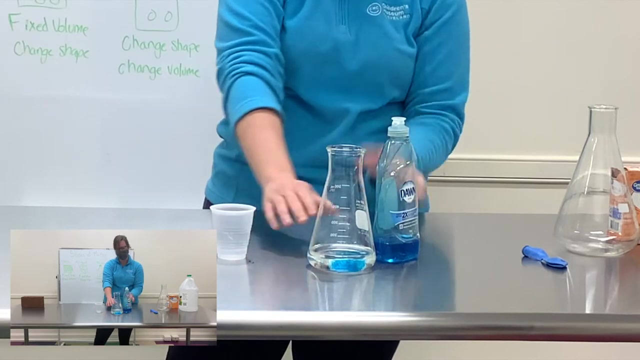 So my soap is a liquid, but it is more viscous or a little bit thicker And, just like the water, it has taken the shape of its container. So liquids have a fixed amount but take the shape of their container. Our third state of matter is a gas, And to demonstrate gas we're going to try an experiment. 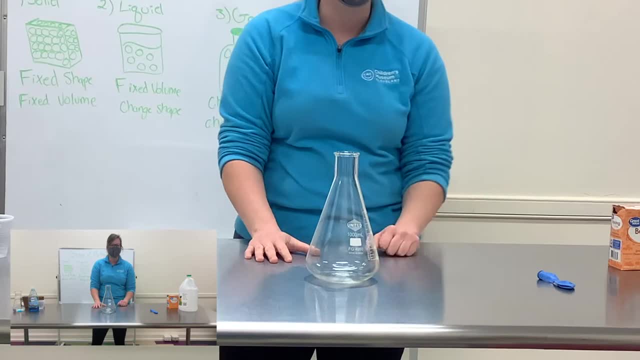 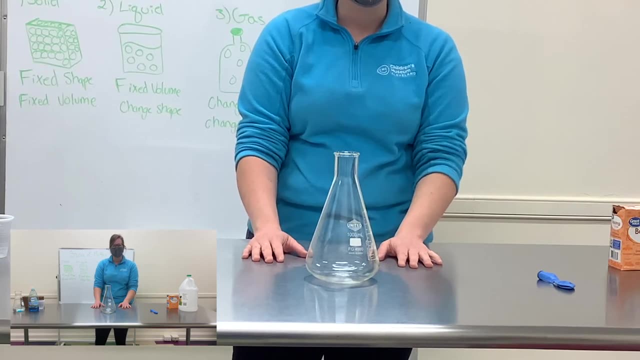 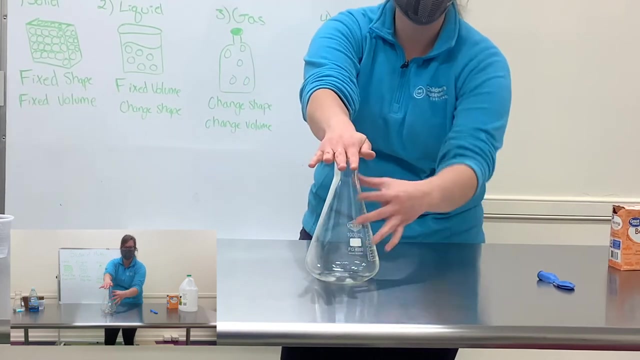 real quick that you could try at home. So gases are different than solids and liquids in that they do not have a fixed shape or a fixed volume. So if I trapped the gas inside this container, it would stay this amount of gas, the same volume as the container, and it would stay this amount of. 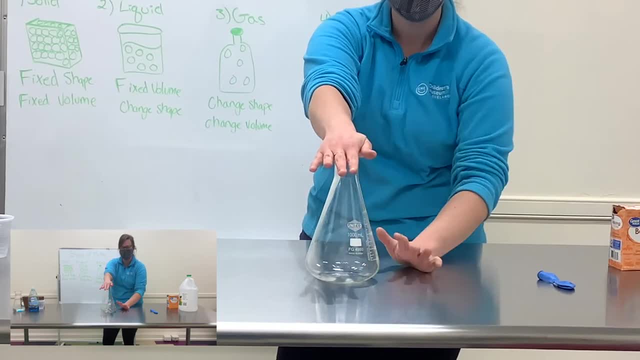 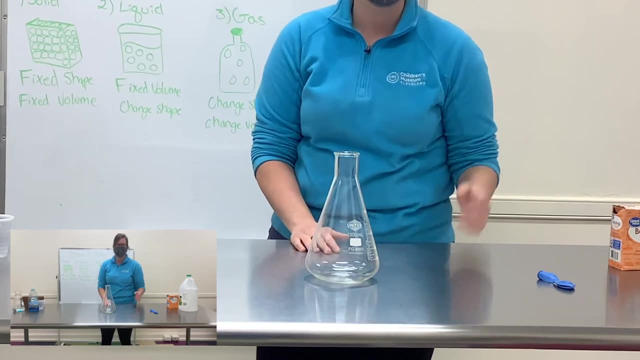 gas the same volume as the container. If I let the gas release it would take up the entire space I'm in, So its volume would change and it also does not have a definite shape To make a gas. today I'm going to do a simple. 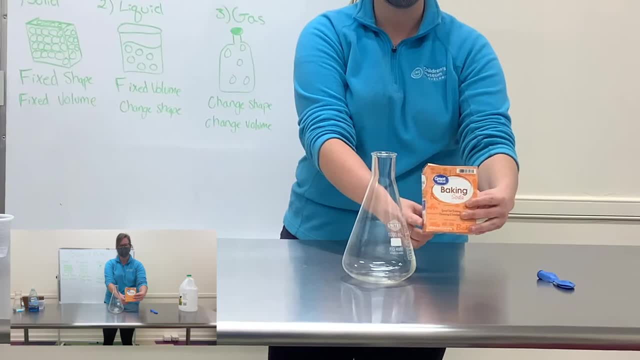 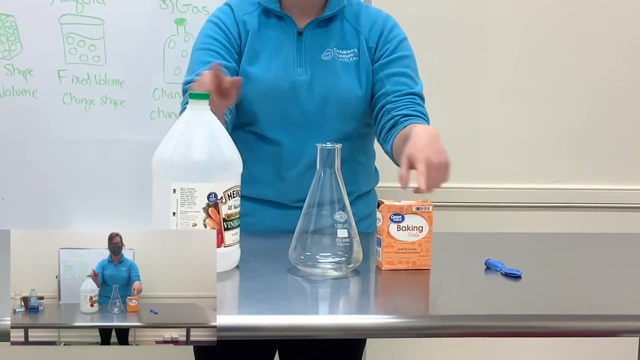 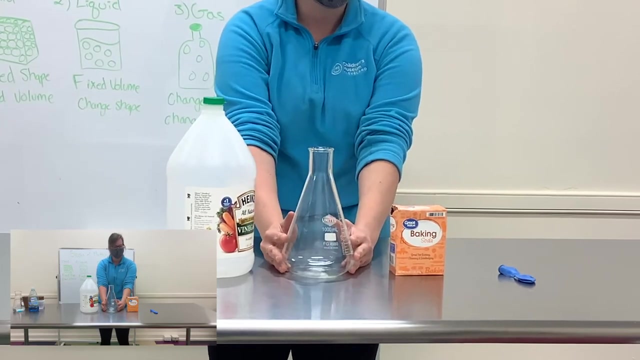 chemical reaction. I'm going to use my solid baking soda and my liquid vinegar, And when I combine the two, we're actually going to have a chemical reaction that produces CO2. Our carbon dioxide, And because gases are often clear, I'm going to put this balloon on the top.